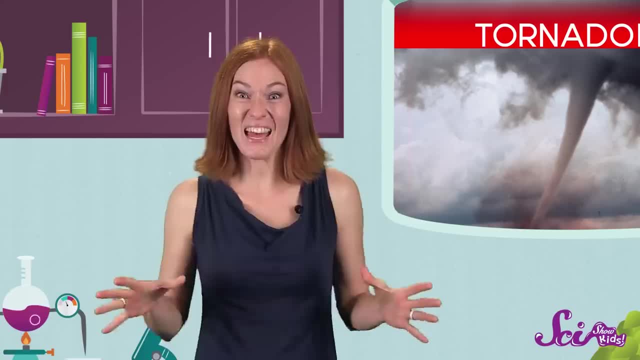 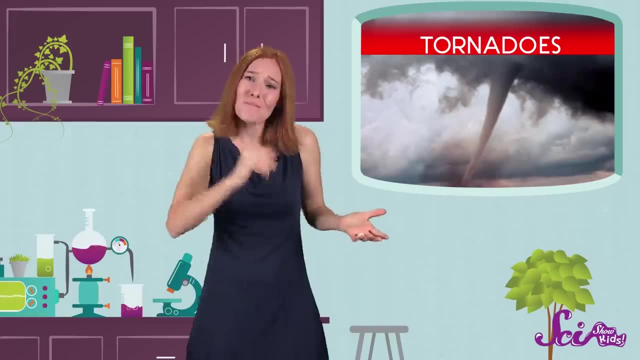 enough to lift heavy things like cars and trucks into the air, And they're loud too. People who have seen them or even been in them say they sound like giant roaring trains, But they don't move as fast as a speeding train. Usually, tornadoes travel across the. 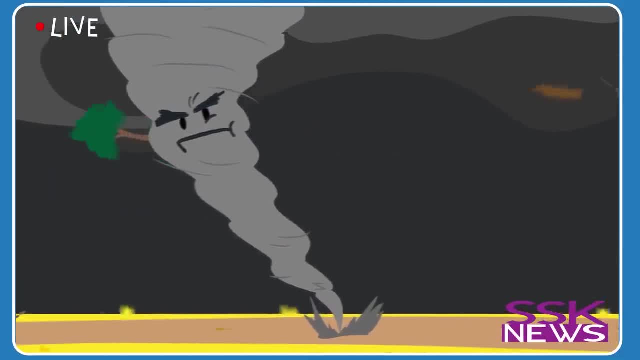 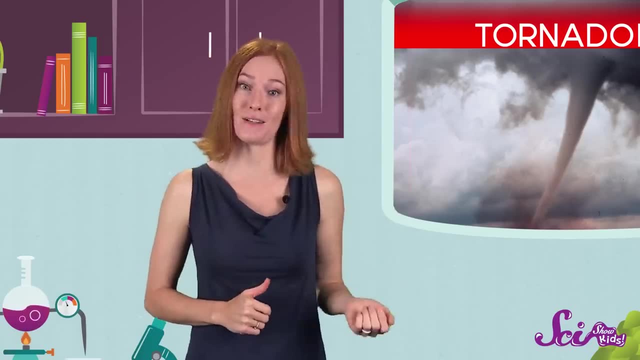 land at about 50 kilometers an hour, slower than most cars go Now. weather can be really unpredictable, which means that you just can't predict or know what's going to happen before it happens, And that's especially true for tornadoes. 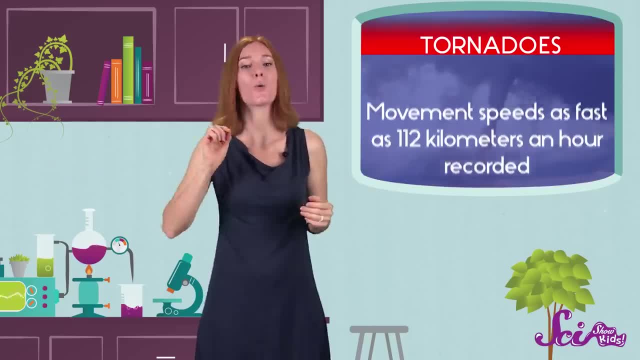 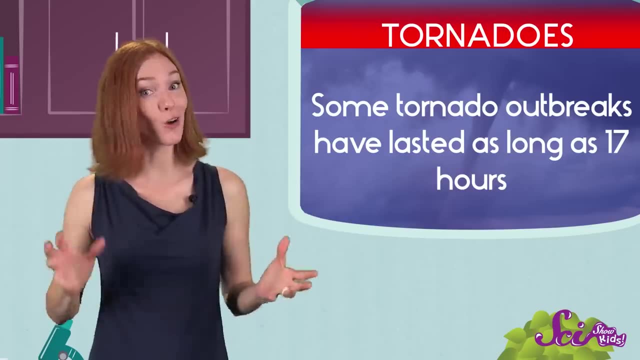 These windy storms can speed up, slow down, change direction or even stand still, And they can last anywhere from a few seconds to as long as an hour. While tornadoes can happen all over the world, they're most common in the United States. 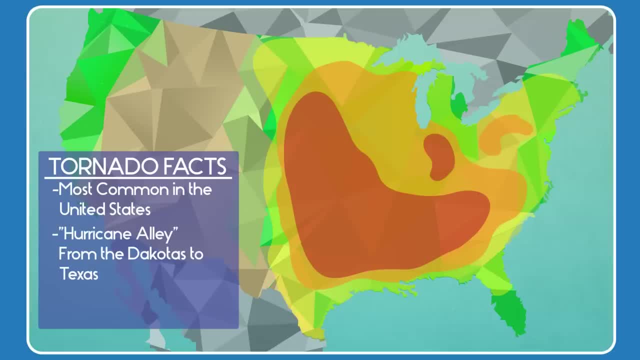 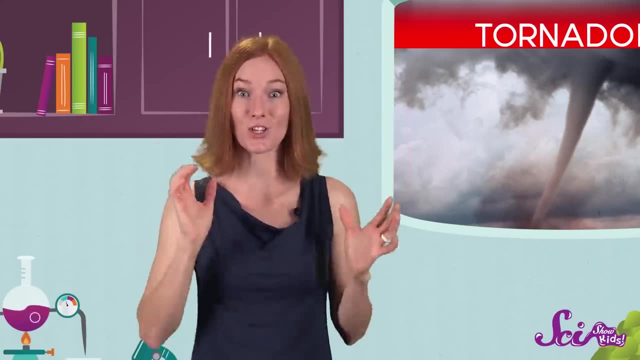 About two-thirds of all the tornadoes in the world happen right down the middle of the country, from the Dakotas down to Texas, Especially in the late spring and early summer. Because tornadoes are so powerful and so unpredictable, meteorologists spend a lot of time studying. 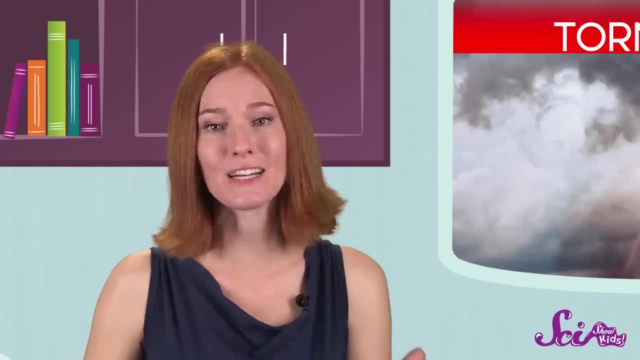 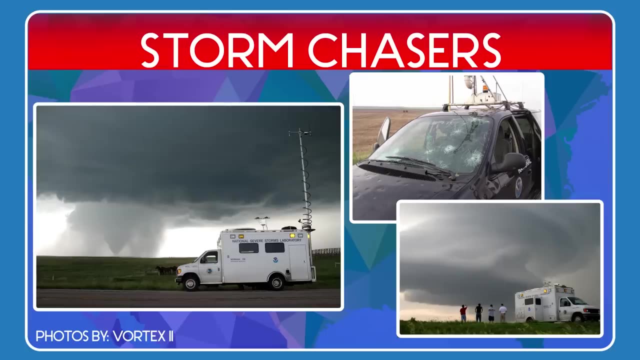 them. They want to understand more about exactly how and when tornadoes can form and hopefully predict when they'll show up. There are even people called storm chasers, who follow big storms around the middle of the US, hoping to spot one as it turns into a tornado, so we can get a better picture. 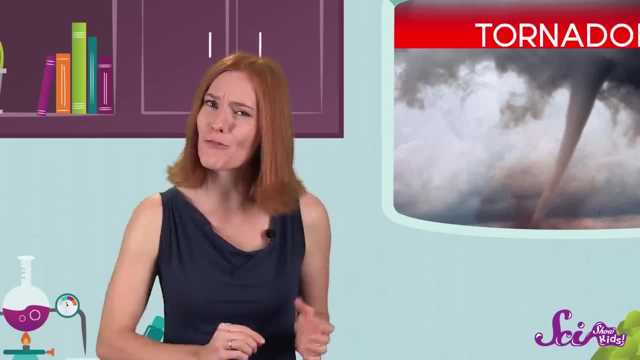 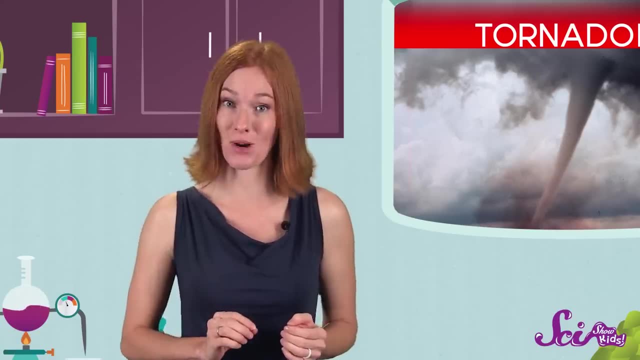 of what really happens when a twister forms. Scientists still don't know for sure when a tornado is going to happen, But they have gotten better at predicting which thunderstorms might be strong enough to create one, And if they spot a bad-looking storm early enough, then they can give people who live. 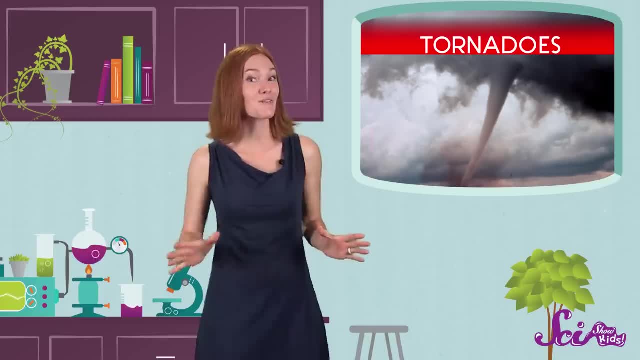 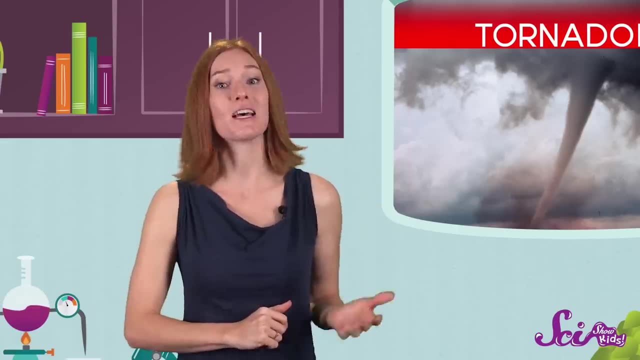 nearby a warning that a twister might be coming. That's one of the most important jobs that a meteorologist has: helping people get ready for extreme weather. So the more they learn about tornadoes, the better we can prepare for them And the more they can help us understand how our weather works, even when it's not so. 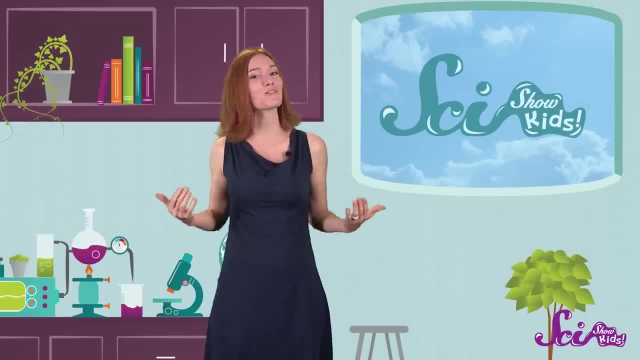 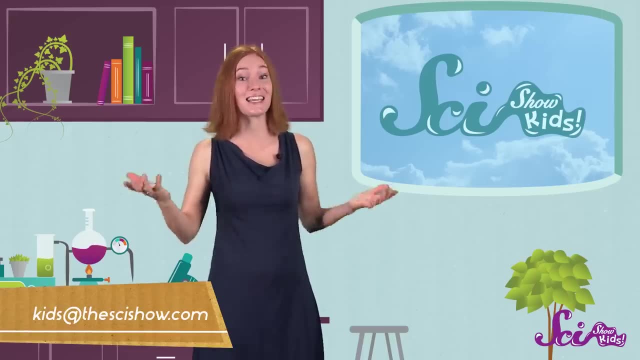 extreme. I hope the weather is nice where you are. If you have any questions for any of us here at the Fort about weather, animals, space or anything, just let us know by leaving a comment or emailing us. at kids at the scishow. dot com. Thanks for joining us and see you next time.